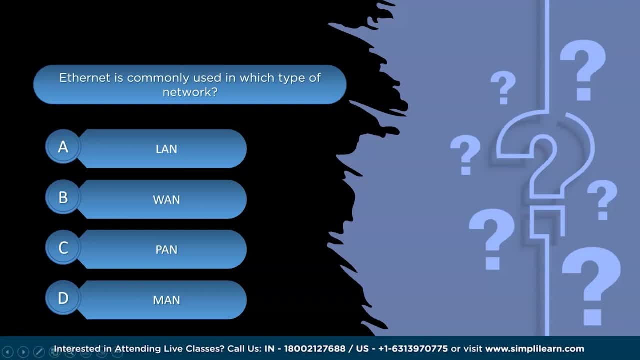 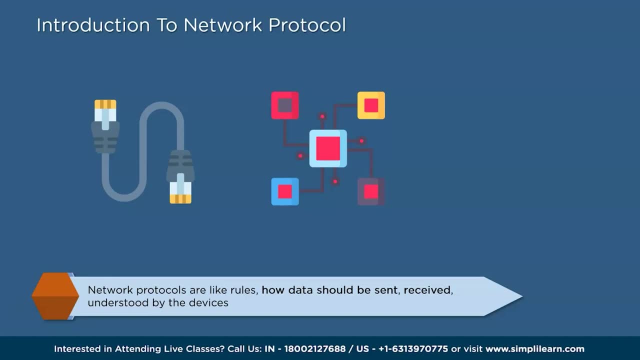 Now you can pause this video and answer in the comment section below. So let's start with the first topic, which is introduction to network protocol. A network protocol is like a set of rules that govern how devices in a network communicate with each other. 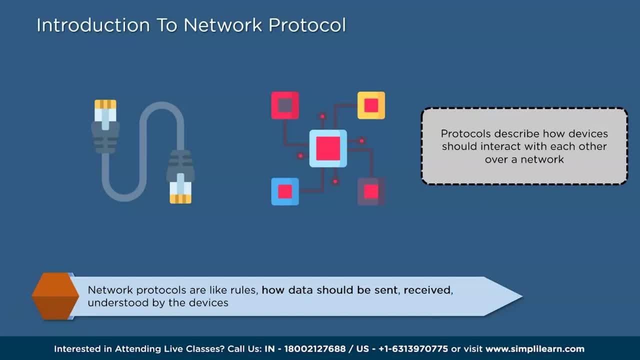 These rules are like instructions that specify how data should be sent, received and understood by the devices. Network protocols are formalized requirements and plans that consist of rules and procedures that describe how devices should interact with each other over a network. They provide a communication system to exchange information using various physical means, such 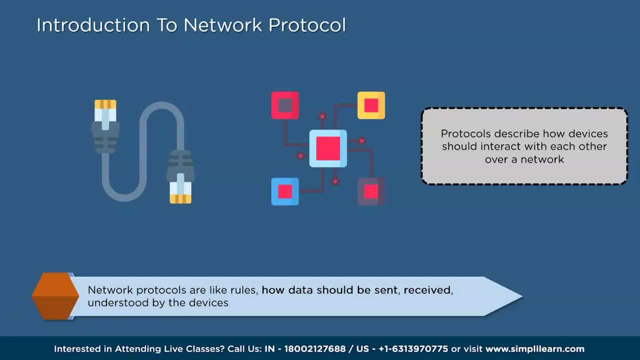 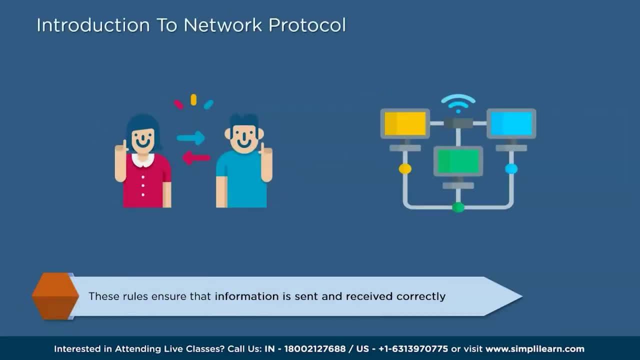 as cables or wireless connections. Just like humans follow certain protocols when they interact with each other, network protocols define a specific steps and guidelines for devices. These rules ensure that information is sent and received correctly and all devices involved understand each other. In essence, network protocols are a way for devices to speak the same language and follow. 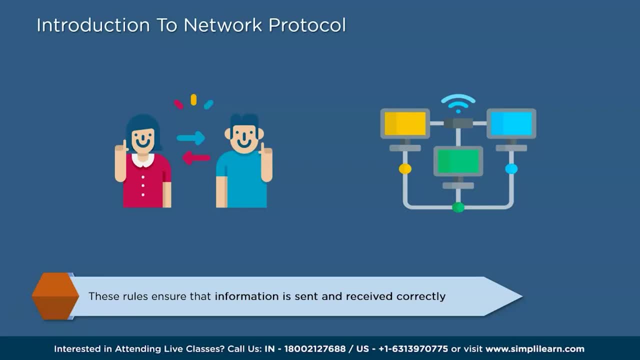 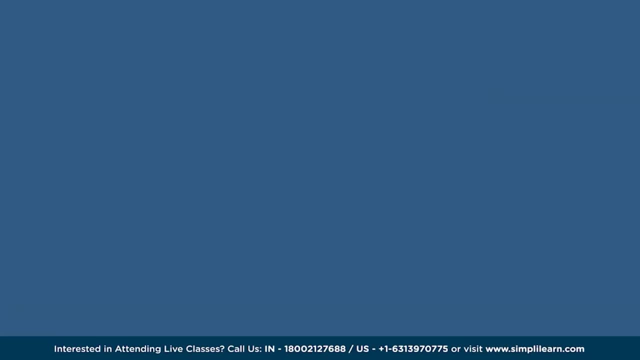 a common set of guidelines so that they can successfully share information and work together effectively. Now let's understand the need of network protocols. Alright, so let me explain this to you in simple terms. Network protocols are like guidelines that devices follow when they communicate with. 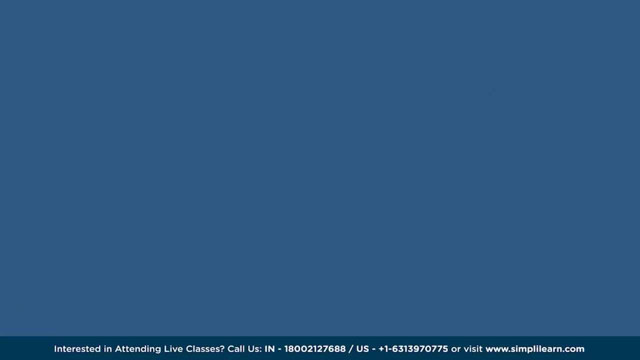 each other over a network. protocols are needed for several reasons. Firstly, network protocols ensure that devices understand each other. Imagine if you and your friend were speaking different languages and had no way to understand each other. Communication would be impossible. Similarly, devices from different manufacturers and with 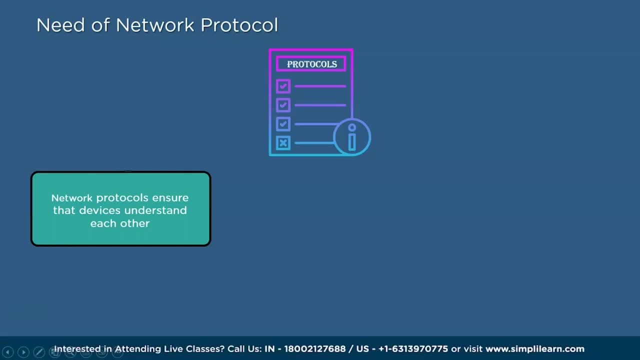 different functions need a common language or protocol to understand each other, signals and data. Secondly, network protocols ensure that data is transmitted reliably. When you send a message or a browser, a website, you want to make sure that the information reaches its destination accurately and 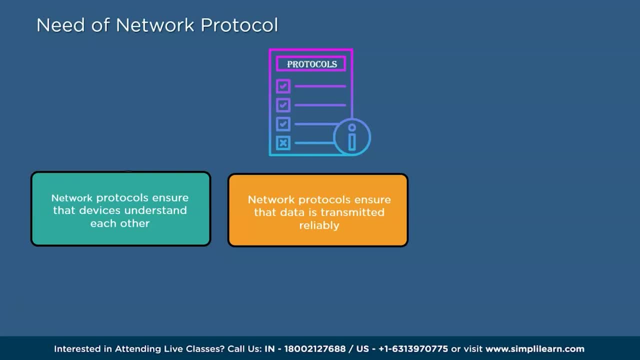 without errors. Network protocols help in breaking down data into smaller packets, sending them across the network and reassembling them correctly at the receiving end. Thirdly, network protocols provide security. They include measures to protect data from unauthorized access and ensure that sensitive information. 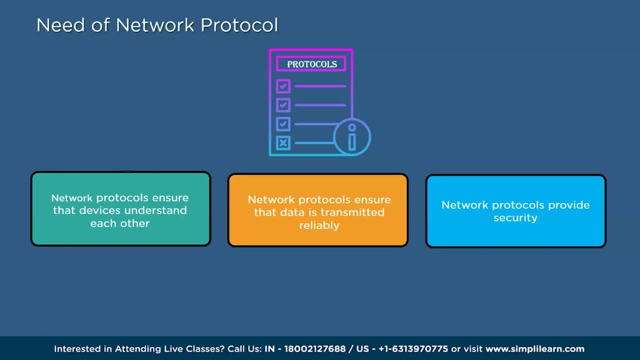 remains confidential. This is particularly important when you make online transactions. Lastly, network protocols allow for interoperability. This means that devices from different manufacturers and with different functions can work together seamlessly. For example, your computer can connect to a printer and your smartphone can access a Wi-Fi network, because they follow the same protocols. 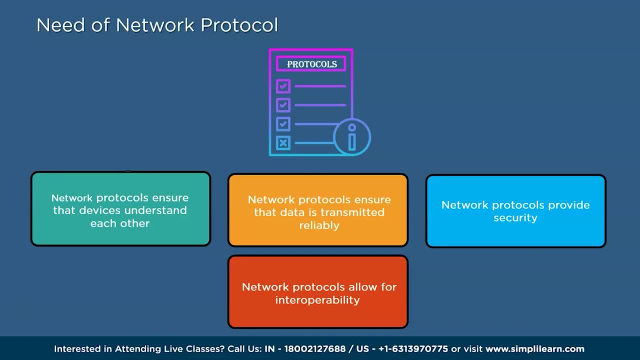 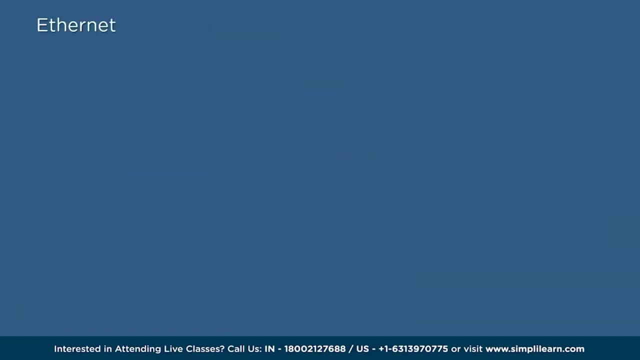 So these were some of the needs of network protocols. Now, before understanding the types of network protocols, we must understand about Ethernet. So Ethernet is a network protocol that is used to connect to the internet. Ethernet is a type of network protocol that helps devices connect and 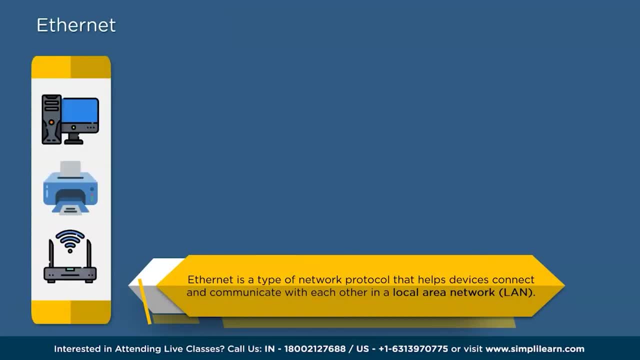 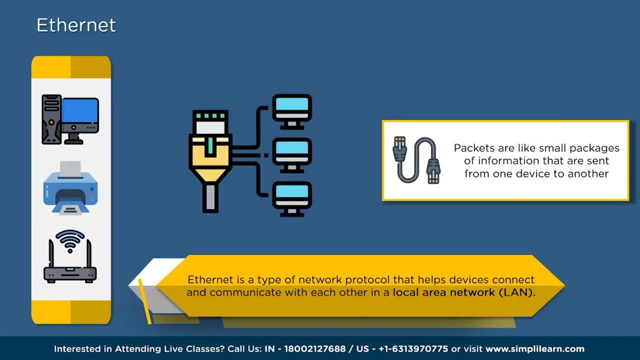 communicate with each other in a local area network, LAN. It is like a highway that allows data to travel between devices such as computers, printers and routers. Ethernet uses a set of rules and procedures to transmit data in the form of packets. These packets are like small packages of information that are sent. 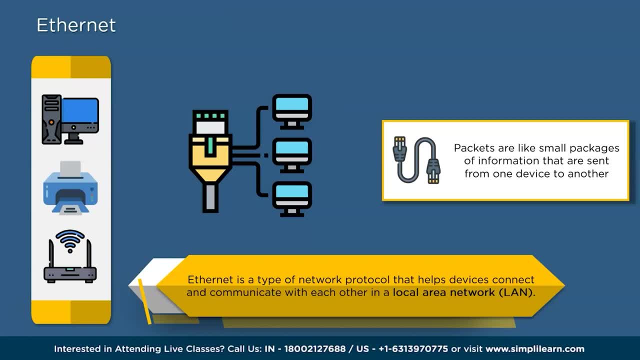 from one device to another. Ethernet ensures that these packets are delivered to the right destination and in the correct order. Think of Ethernet as the system that connects all the devices in a network. It ensures that data can flow smoothly between devices, enabling them to share information and work together. 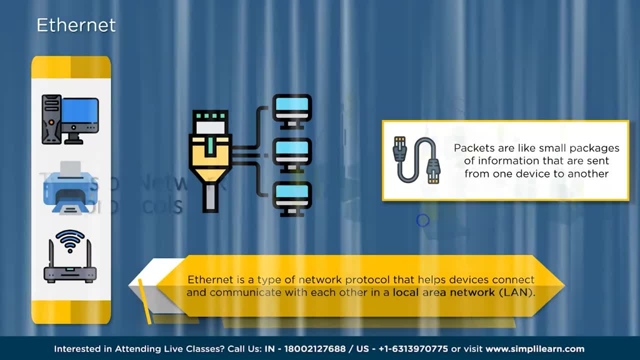 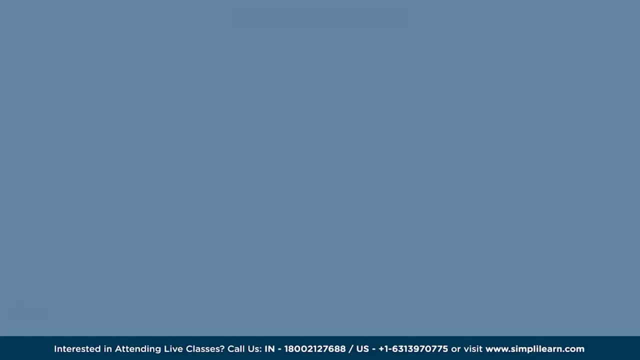 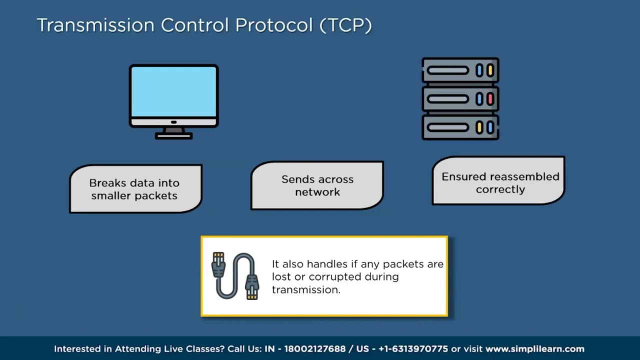 efficiently. Now let's have a look at the types of network protocols. Here we will cover some of the types of network protocols. We'll start with the first one, which is TCP, that is, transmission control protocol. TCP is a network protocol that ensures reliable and order delivery of data between devices. It 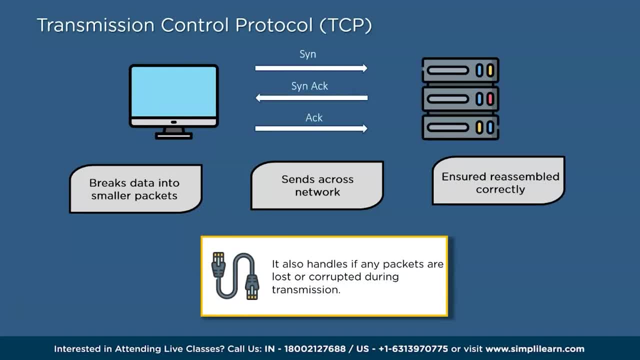 breaks down data into smaller packets, sends them across the network and ensures that they are reassembled correctly at the receiving end. TCP also handles error detection and retransmission if any packets are lost or corrupted during transmission. So this was about TCP or transmission control. 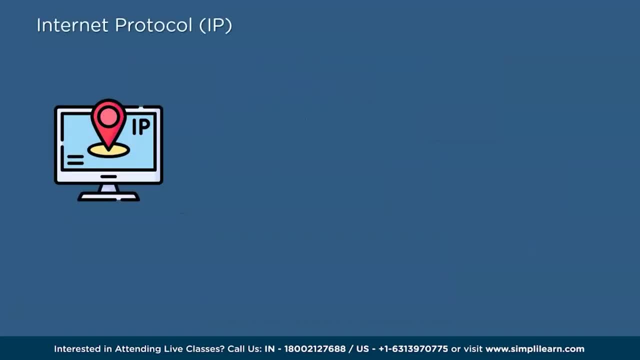 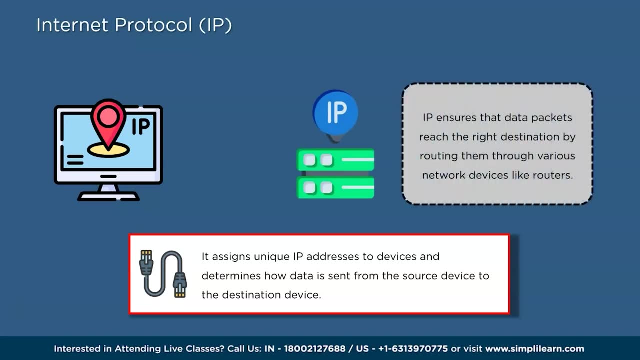 protocol. Now, second is IP, that is, internet protocol. IP is another network protocol that handles the addressing and routing of packets across the internet. It assigns unique IP addresses to the network. It also shifts data addresses to devices and determines how data is sent from the. 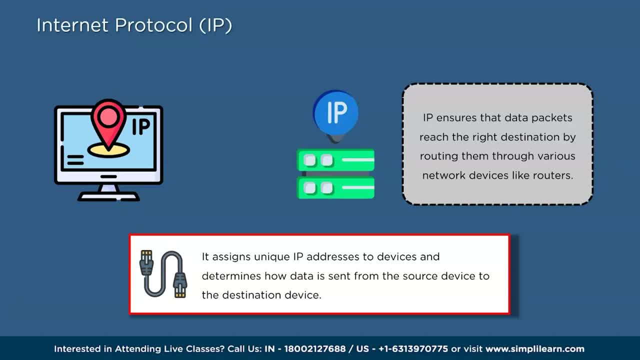 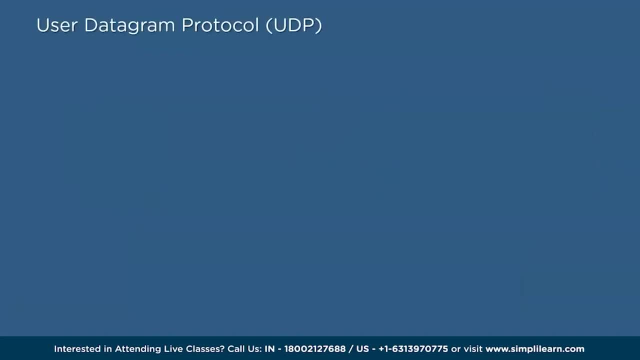 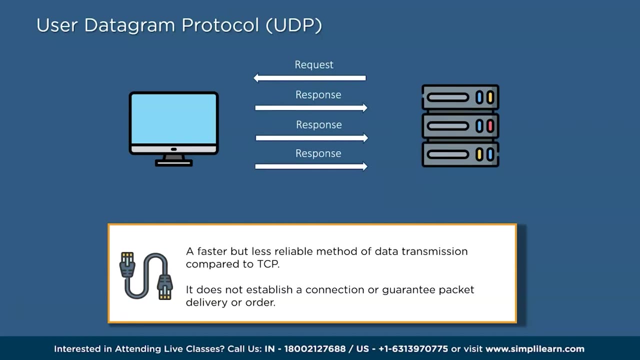 source device to the destination device. IP ensures that the data packets reach the right destination by routing them to various network devices like routers. Third is UDP or user datagram protocol. UDP is a network protocol that provides a faster but less reliable method of data transmission compared to TCP. It does not 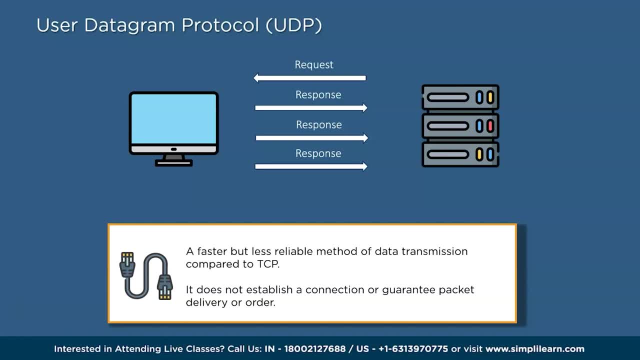 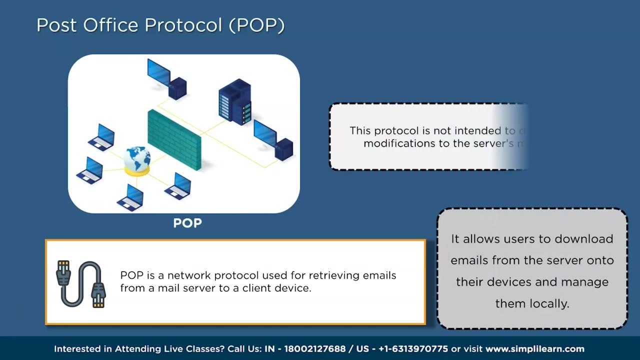 establish a connection or guarantee packet delivery or order. UDP is commonly used like video streaming or online gaming, where a small amount of data loss is acceptable. next is POP, that is, post office protocol. POP is a network protocol used for retrieving emails from a mail server to a client device. it 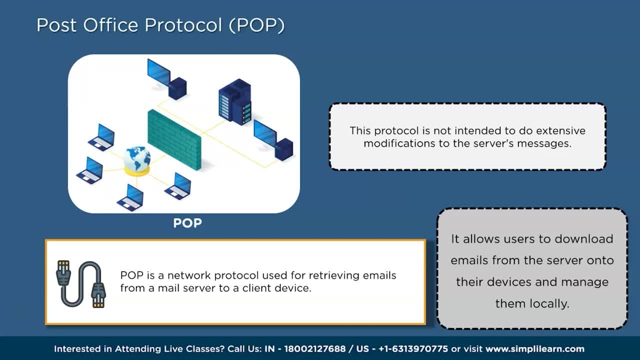 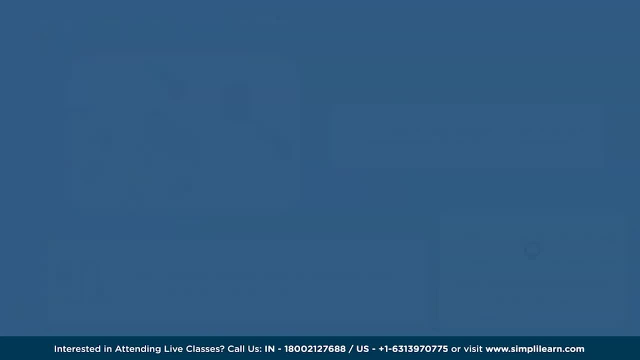 allows users to download emails from the server onto their device and manage them locally. POP is typically used by email clients like Outlook or Thunderbird. next we have is SMTP, or simple mail transfer protocol. SMTP is a network protocol used for sending emails from a client device to a mail server. it handles the 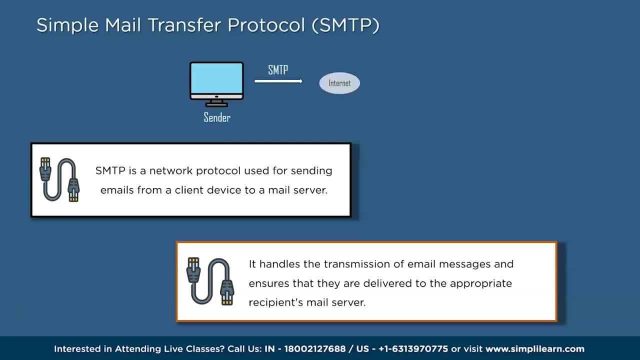 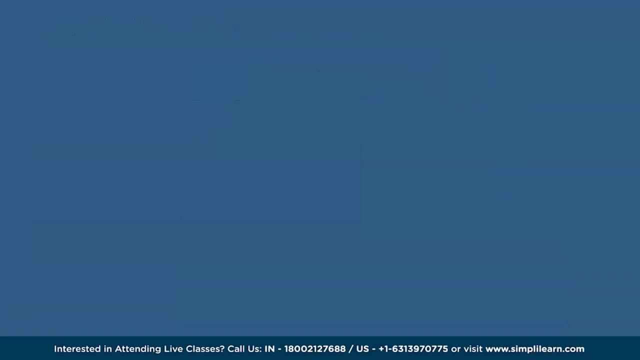 transmission of email messages and ensure that they are delivered to the appropriate recipients. mail server SMTP is responsible for the reliable transfer of email across different mail servers. so this was about simple mail transfer protocol. now let's understand the sixth one, which is file transfer protocol, or FTP. 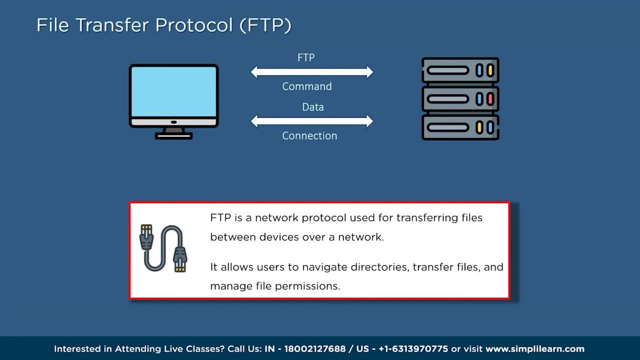 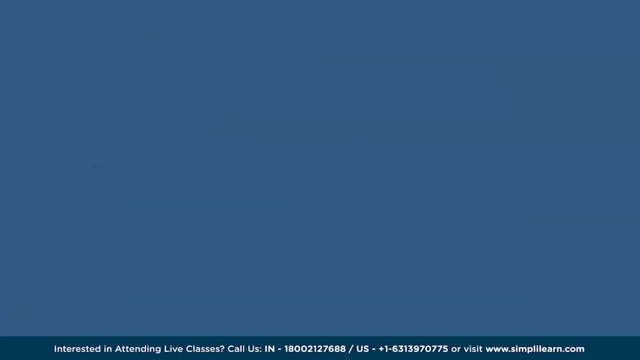 FTP is a network protocol used for transferring files between devices over a network. it provides a standard method for uploading and downloading files to and from a remote server. FTP allows users to navigate directories, transfer files and manage file permissions. now coming to the next, which is hypertext. 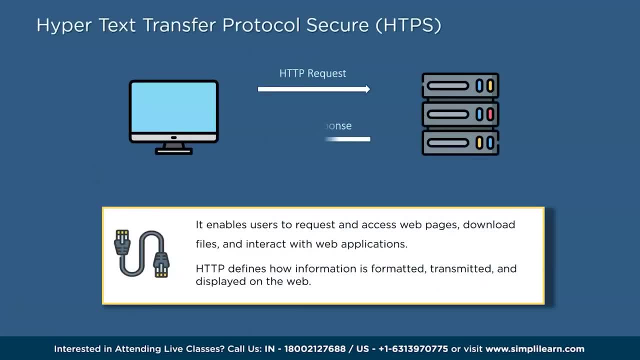 transfer protocol secure, that is HTTPS. HTTP is a secure version of HTTP that provides encryption and authentication. it ensures that the data transmitted between a web browser and a web server is encrypted and protected from unauthorized access. HTTPS is commonly used for secure online transactions, sensitive data transfers and protecting users privacy. so these 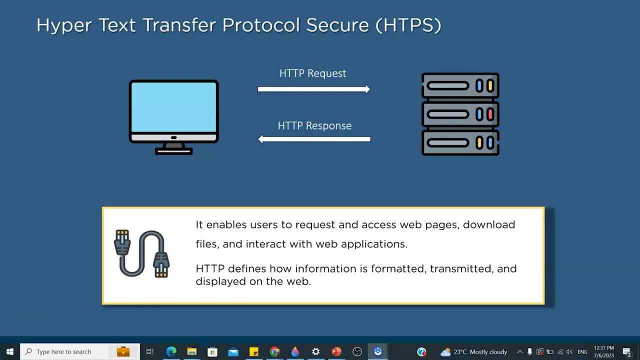 were some of the types of network protocols. so basically, network protocols- rare, crucial role in enabling communication and data transfer across various computer networks. we have explored several types of network protocols, each serving specific purpose and operating at different layers of network. ¿dose trabajar en diferentes businesses y蛋 competition tendria interogran specialne en opera salted cables y Ahhh sort deanutes perspectiva deaiah network ab Juda y districts plataformas entani han photons que ejė transcribir-se de Facebook. network protocols, each serving specific purpose and operating at different areas of networking address. 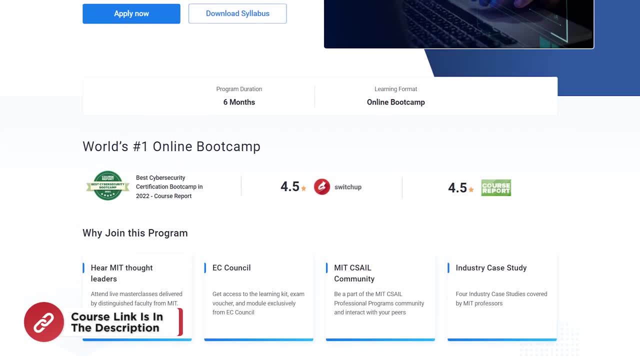 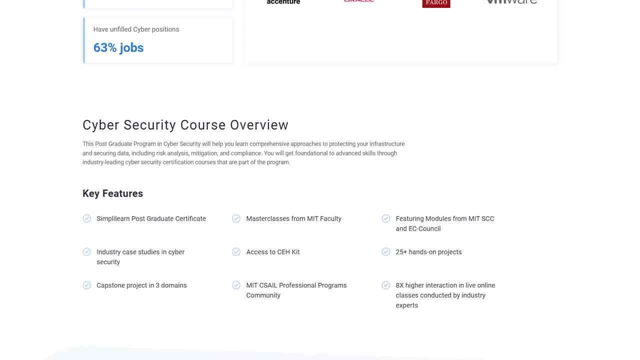 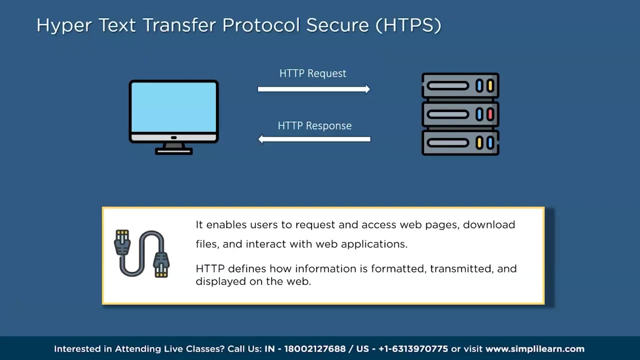 order. So if you are someone who is interested in building a career in cybersecurity by graduating from the best universities, then try giving a shot at Simply Learn's postgraduate program in cybersecurity with modules from MIT Schwarzman College of Engineering. Also have a look at what a learners has to.